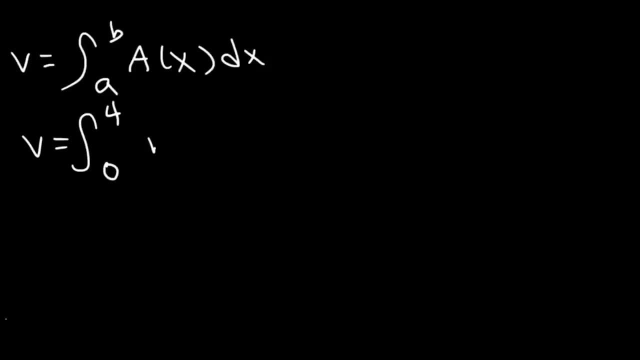 0 to 4 and a of x is simply x the antiderivative of x is x squared divided by 2 evaluated from 0 to 4 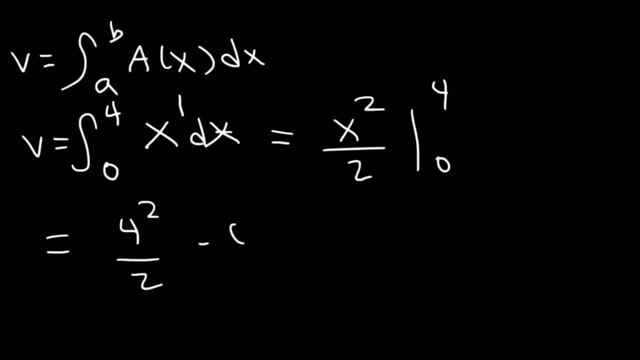 so first let's plug in 4 x squared divided by 2 so first let's plug in 4 and then we will plug in 0 4 squared is 16 16 divided by 2 is 8 so that is the answer 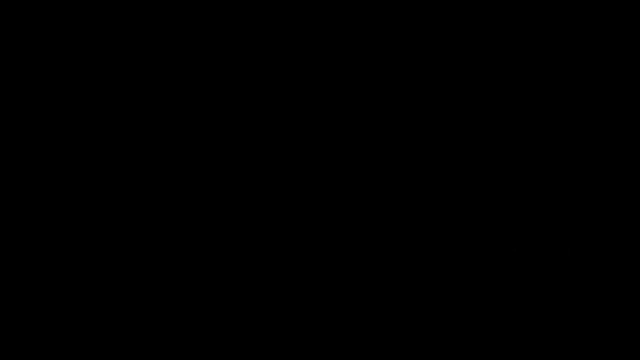 now another way in which you can graph this particular problem 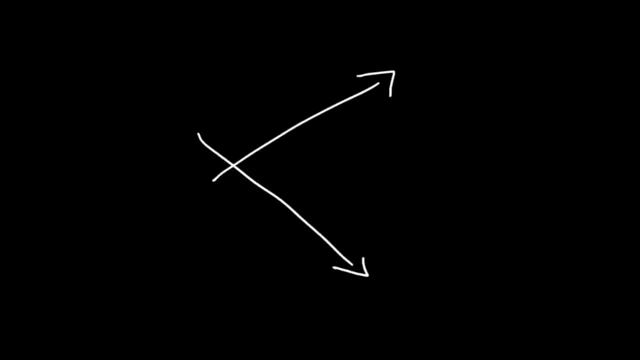 is you can draw it like this if you want to see why we set it up the way we did 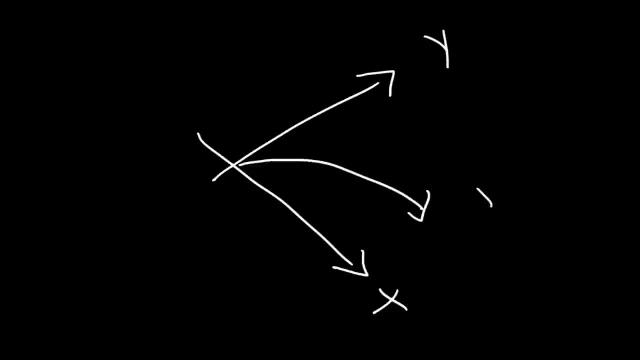 so this is the graph y equals square root x and we said this that line is basically s 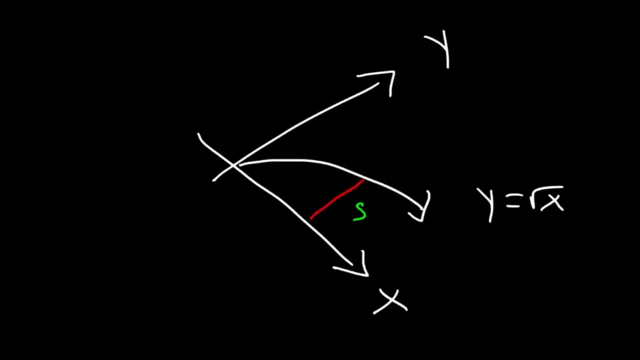 it represents the base of the square and let's draw the square so there is a square you can draw it that way too and so this is s as well 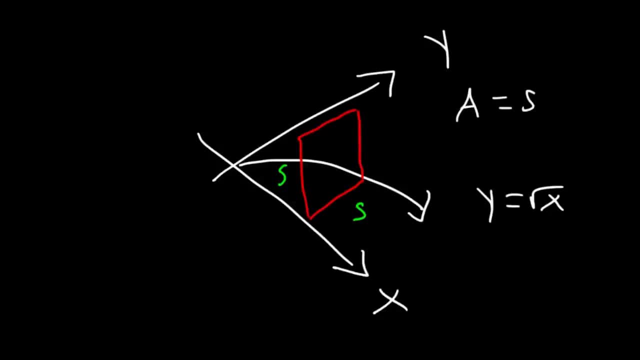 and so you can see that the area is s squared and you can also see that y is equal to s so you can graph it that way it may help you to understand that to visualize it better 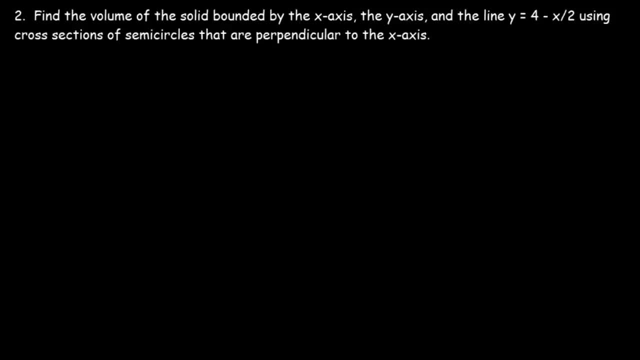 number two find the volume of the solid bounded by the x axis the y axis and the line y equals 4 minus x over 2 using cross sections of semi circles that are perpendicular to the x axis so if the cross sections are perpendicular to the x axis ultimately we need to use this equation to find the volume so we are going to use this equation to find the volume So we've got to find the area of the cross-section in terms of x. But now let's go ahead and graph the equation. 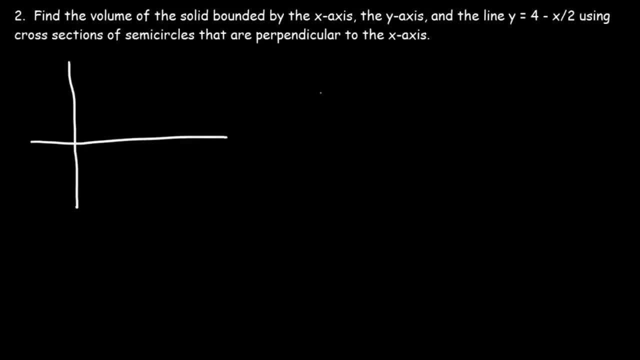 So we have a line, which is 4 minus x over 2. We can rewrite it as negative 1 over 2x plus 4. So now it's in a slope-intercept form. So the slope is negative 1 half, and the y-intercept is 4. So we could graph it at the point 0, 4. And if the slope is negative, it's a decrease in function. Now let's find the x-intercept. To do that, replace y with 0. 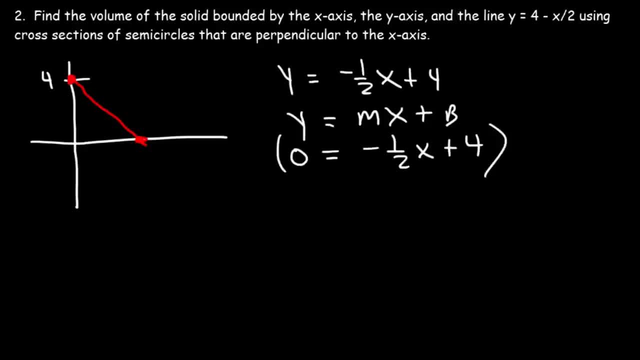 And solve. So we can multiply both sides by 2. Negative half times 2 is negative 1. So this is going to be negative x. 4 times 2 is 8. 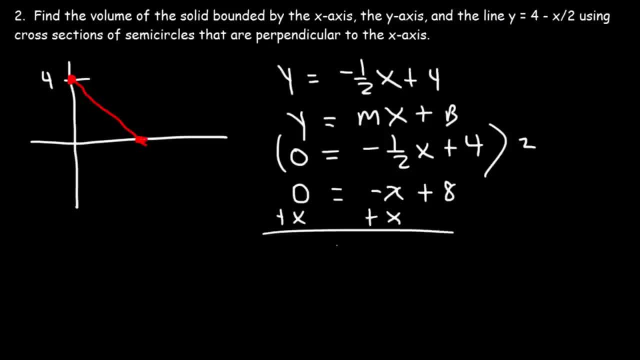 So if we add x to both sides, we see that x is equal to 8. So the x-intercept is 8, and the y-intercept is 4. 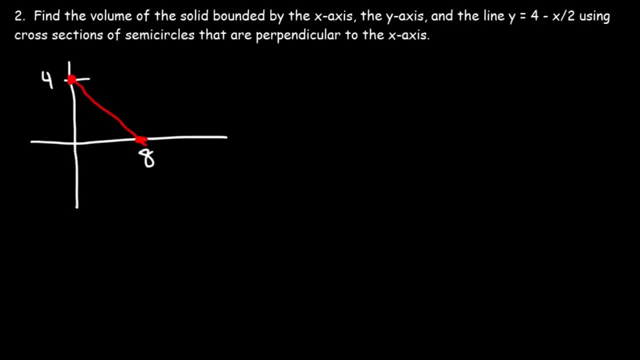 Now the cross-sections are perpendicular to the x-axis. So that means s is parallel to the y-axis. So this is s. Now we can graph the function another way too. 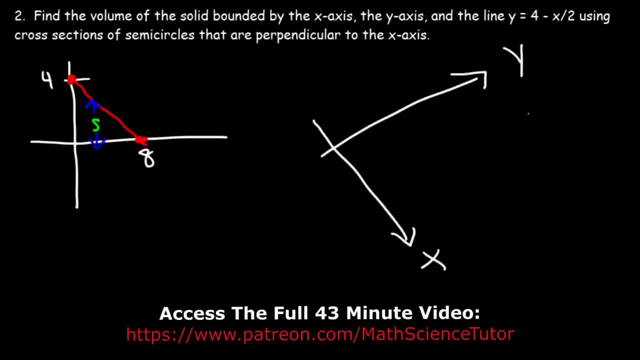 Let's say that's the x-axis. This is the y-axis. And the cross-sections are perpendicular to the x-axis. Which means they're parallel to the y-axis. And they're basically a semicircle. So that's the graph. And this is s. 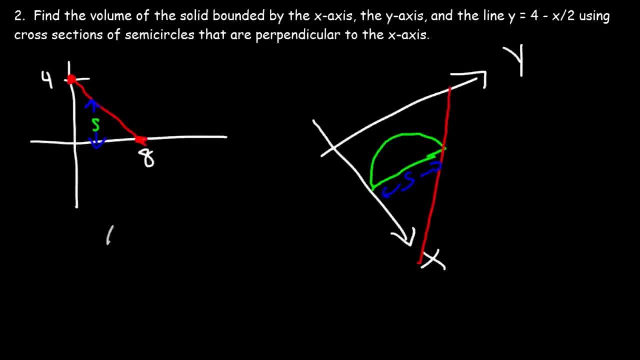 So as you can see, s represents the diameter. Of the semicircle. 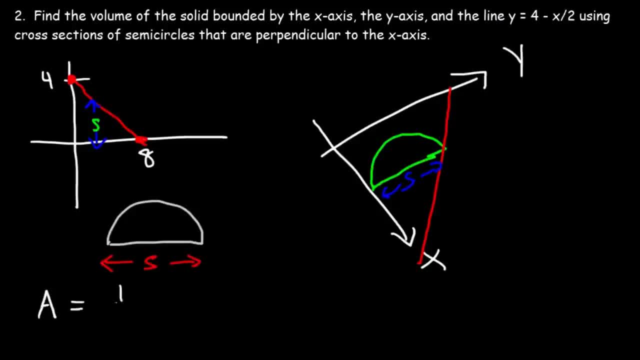 Now we know that the area of a semicircle is 1 half pi r squared. And so the radius is half of s. So s is equal to 2r. And 1 half of s is equal to r. So let's replace r with s divided by 2. So the area is 1 half pi. Times 1 half s squared. 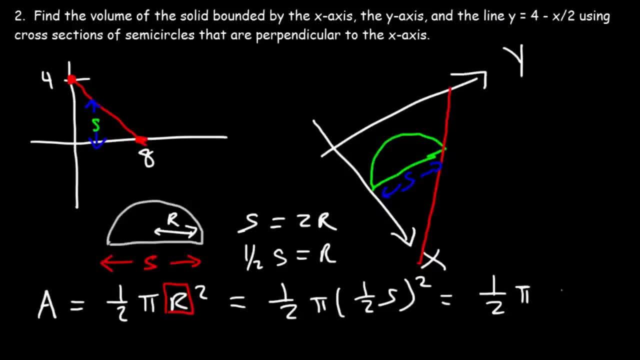 1 half squared is basically 1 fourth. If you do 1 over 2 times 1 over 2, you get 1 over 4. So this is 1 over 4 s squared. So therefore the area is 1 half times 1 fourth is 1 eighth. 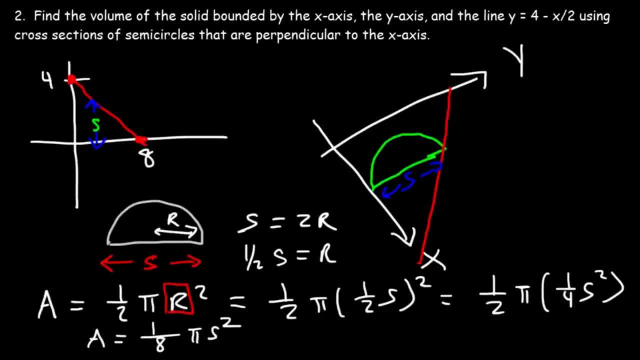 So it's 1 over 8 pi s squared. And if you look at the graph, we can see that s is the same as y. So s equals y. 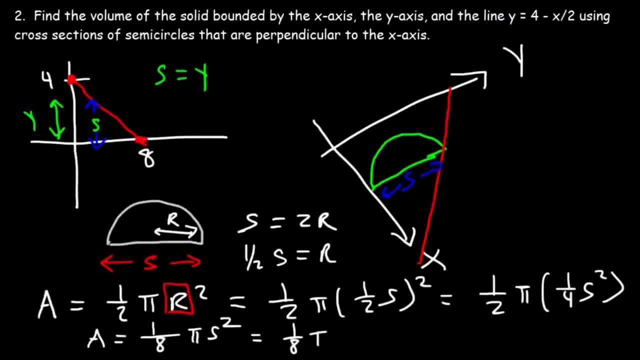 So the area in terms of y is 1 over 8 pi y squared. Now let's get rid of a few things. Let's make some space. 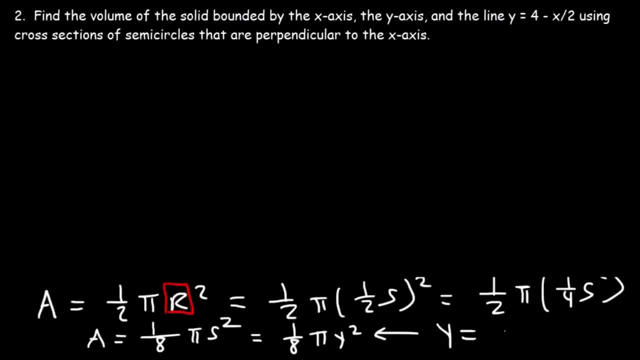 So at this point, we can replace y with 4 minus x over 2. Or let's just use, let's use that. So the area is going to be 1 over 8 pi. Times 4 minus 1 half x squared. So now we have the area function in terms of x. Which means we can now use this equation to calculate the volume. 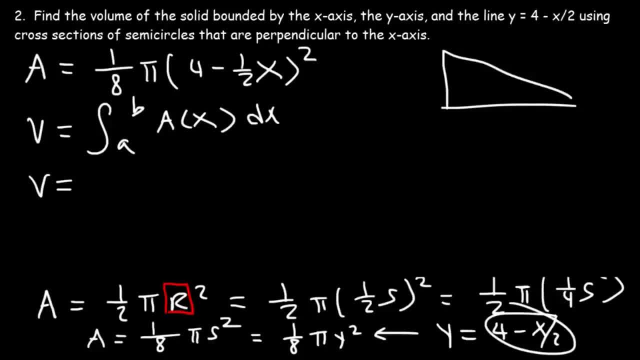 So the graph was bounded between 0 and 8. So a is 0, b is 8. 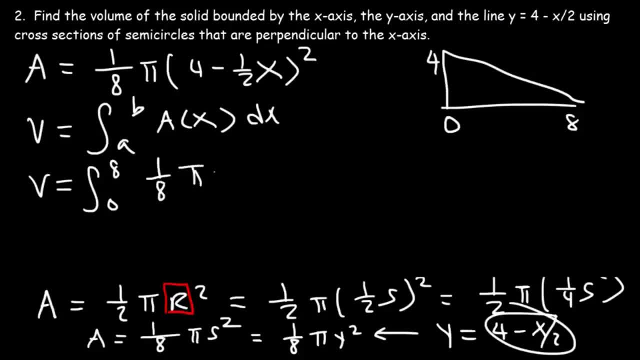 And then we can integrate the area function at this point. And let's not forget dx. 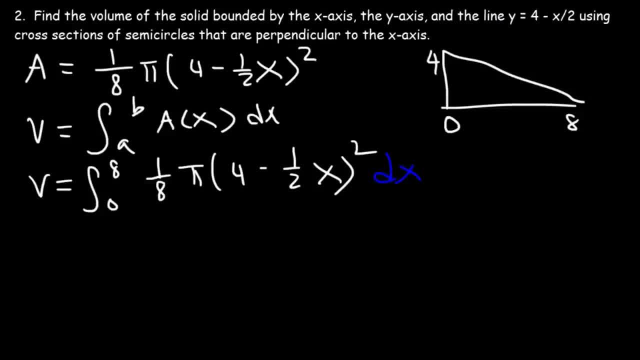 Now before we find the integration of that function, we need to FOIL 4 minus 1 half x squared. So that's 4 minus 1 half x times itself. So 4 times 4, that's equal to 16. And then we have 4 times 1 half x, which is negative 2x. And negative half x times 4 is also negative 2x. And then negative 1 half x times negative 1 half x. That's positive 1 fourth x squared. 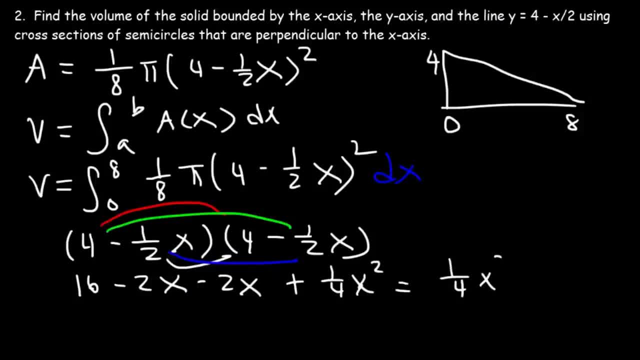 So this becomes 1 fourth x squared. Minus 1 half x. Minus 4x plus 16. If we combine the middle terms. 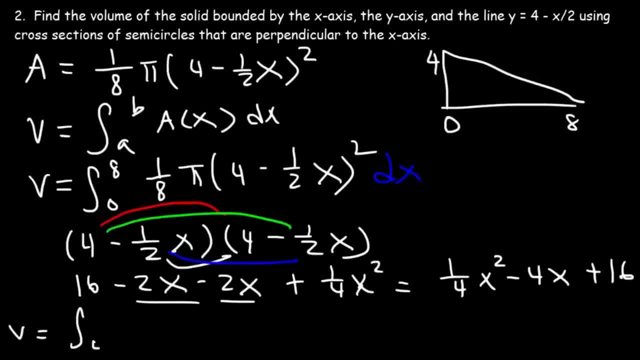 So therefore, the volume is the integration from 0 to 8. 1 over 8 pi. 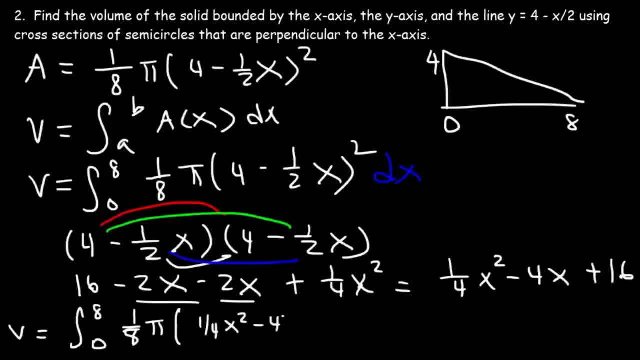 1 fourth x squared. Minus 4x plus 16 dx. 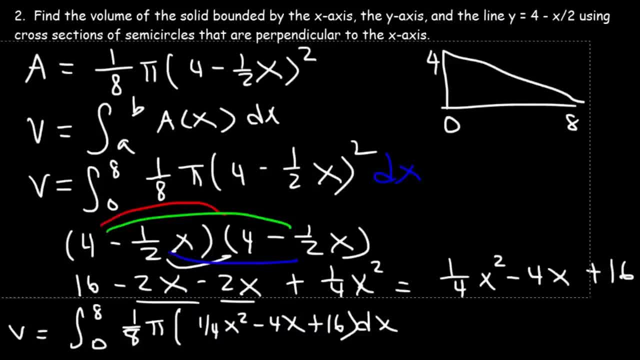 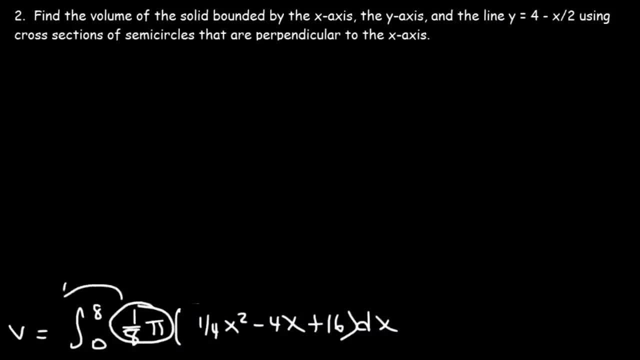 So now let's take the constant and move it to the front. 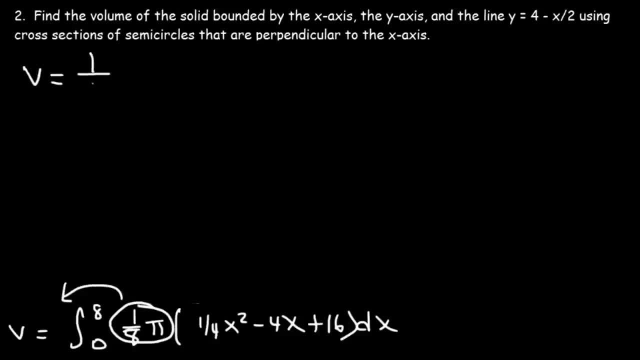 So the volume is 1 eighth pi integration from 0 to 8. 1 over 4x squared minus 4x plus 16 in parentheses with a dx out in the front. So now let's find the antiderivative. 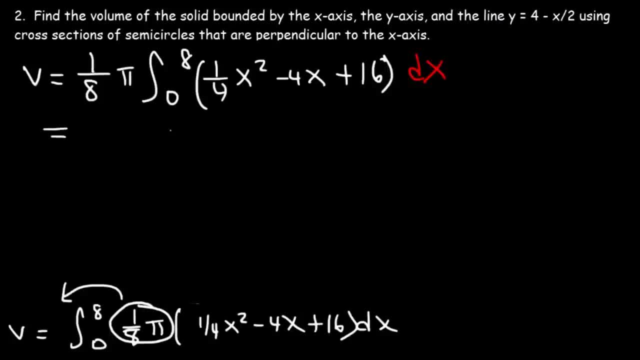 The antiderivative of 1 fourth x squared, that's 1 fourth x to the 3rd divided by 3. The antiderivative of 4x is going to be 4x squared divided by 2. And for 16, it's going to turn into 16x. Evaluated from 0 to 8. 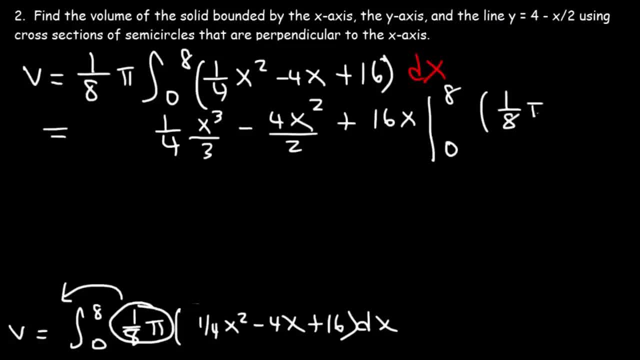 And we still have 1 eighth pi in front. So let's plug in 8. So 4 times 3 is 12. So that's 1 over 12 times 8 to the 3rd power. 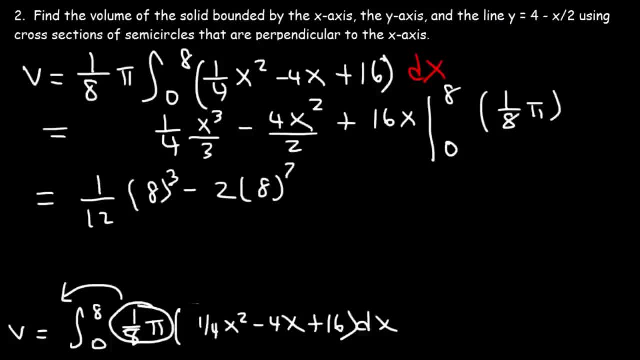 4 divided by 2 is 2. And then we have 8 squared plus 16 times 8. 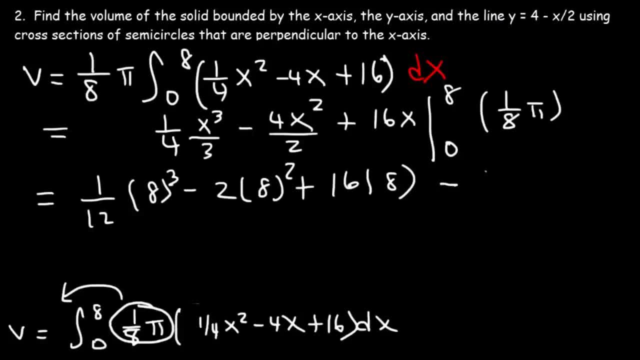 And then minus, we plug in 0 to everything. It's all going to equal 0. 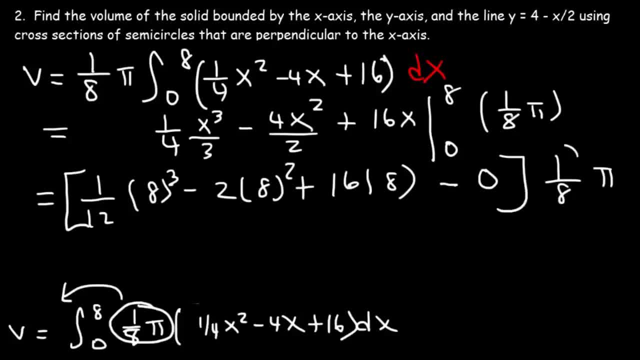 Now what I'm going to do is multiply, or I'm going to distribute the 1 over 8 to every term because they all have 8 inside. 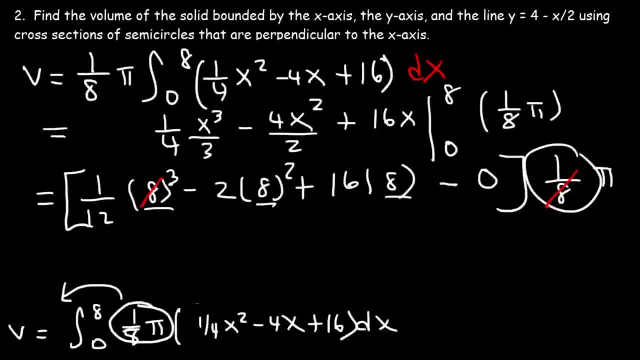 So therefore, this 8 will cancel 1 eighth out of each term that we see there. So that's going to simplify our calculations. 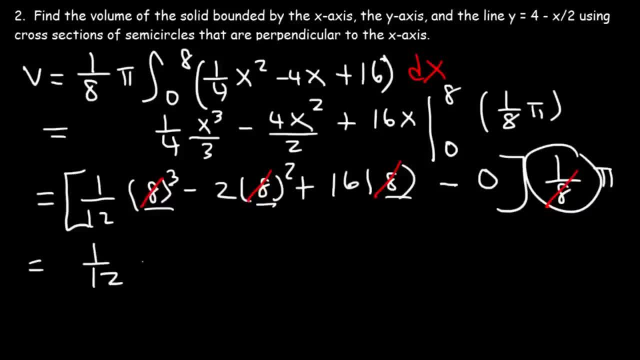 So then this becomes 1 over 12. And instead of 8 to the 3rd, it's now 8 squared. We have to take off an 8. And this is going to be 2 times 8 plus 16. And we're going to have a pi in front now. Negative 2 times 8 is 16 plus 16. Those two will cancel. 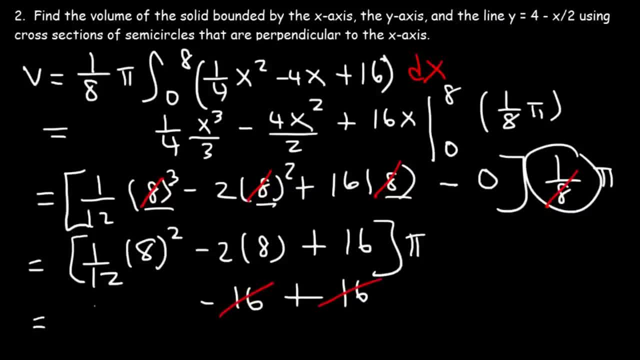 So now we just have this term to deal with. 8 squared is 64. So we have 64 times the pi outside divided by 12. 64 pi over 12. We can reduce it. 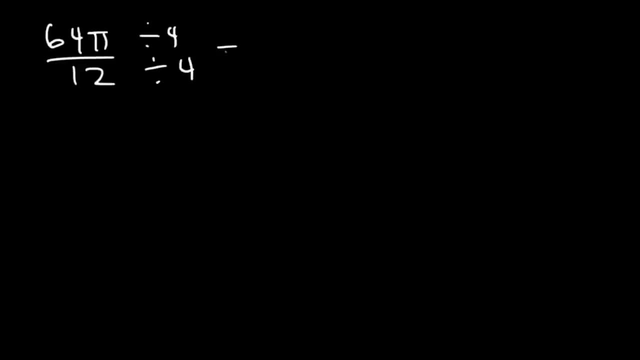 If we divide both numbers by 4, this is going to be 16 pi divided by 3.